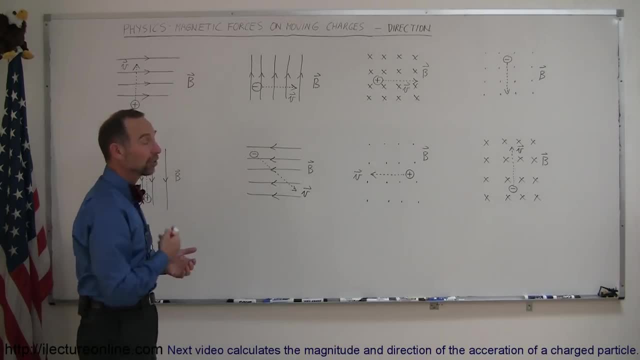 to the direction of magnetic field. So I have a bunch of examples on the board here to try and figure out what the direction of the force will be on each of the charges as they're moving through the magnetic field, Remembering of course that the magnitude of the force can be found by taking 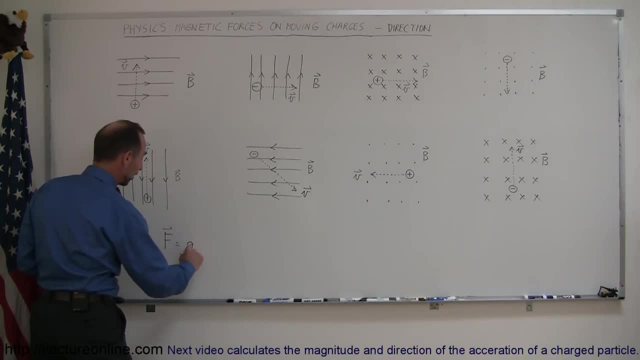 the equation that the force on a moving charge is equal to the size of the charge, q times the current of the charge q. times the current of the charge q times the current of the charge q cross product of the velocity of the charge. times the magnitude of the magnetic field. 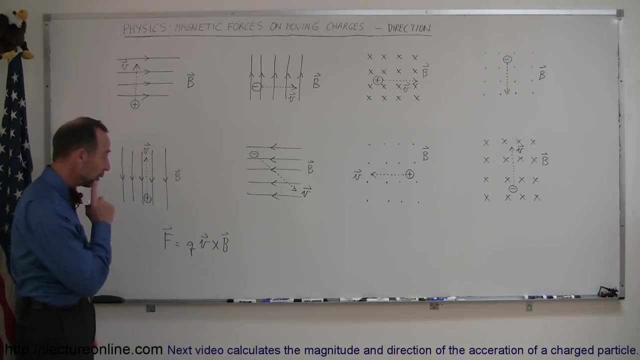 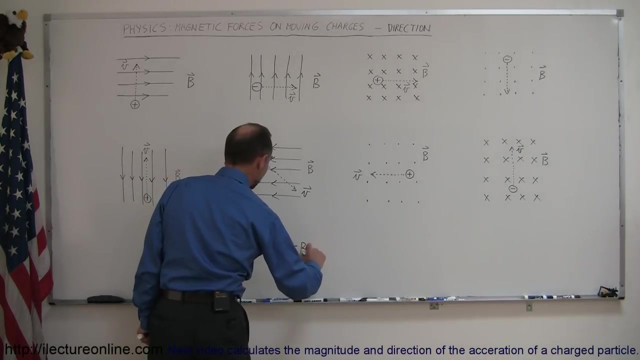 and the direction of magnetic field. so force is q, v cross b and, of course, the. when we want to find the magnitude of v cross b, this can be written as: the magnitude of the force is equal to q times v times b times the sine of the angle between them. now, theta is the angle between the direction of 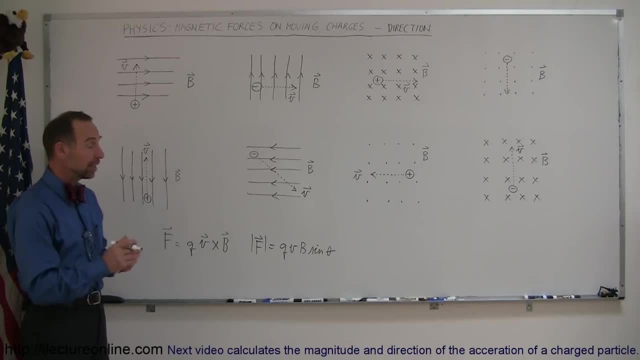 the velocity of the charge and the direction of the b field. and you can see then, if the, if the angle between them is 90 degrees, which means if the direction of the velocity is perpendicular to the direction of the magnetic field, the sine of 90 degrees is one and the magnitude of the 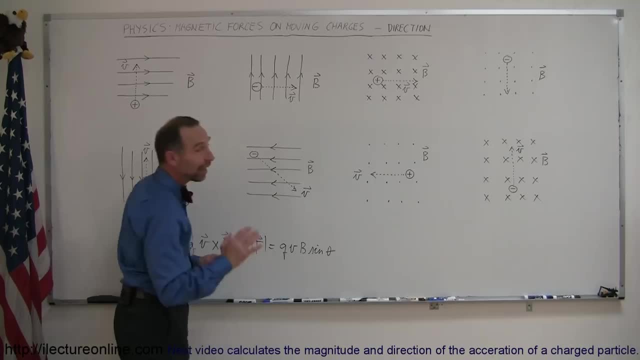 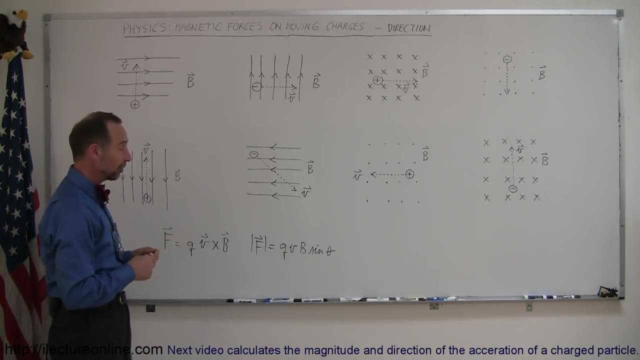 force simply will be q v b. if the angle between them is not 90 degrees, then of course the force will be less than q v b by this factor and of course, if the sine, if the angle is zero degrees between the direction of the velocity and the direction of the magnetic field. 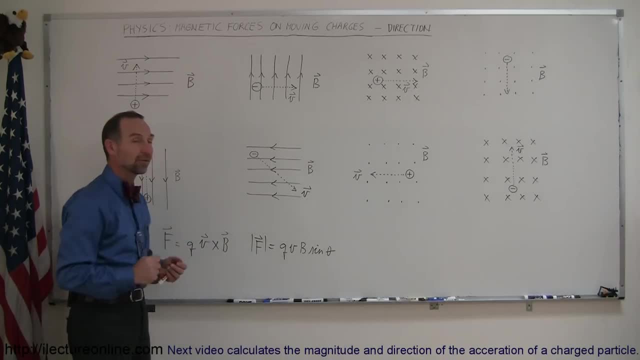 then the force will be less than q v b and the magnitude of the force will be less than q v b, then the sine of zero is zero and the magnitude of force will be zero accordingly. all right, so what we're going to do now is we're going to try and find the direction of the force on each of these. 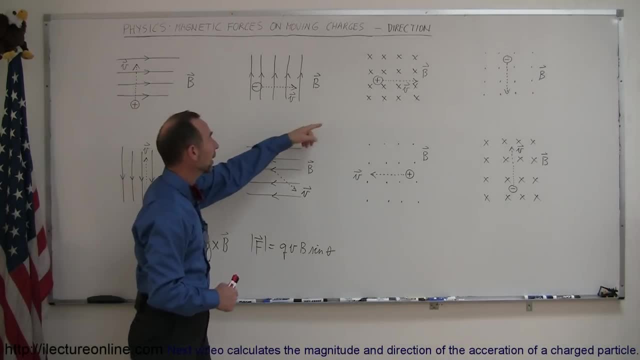 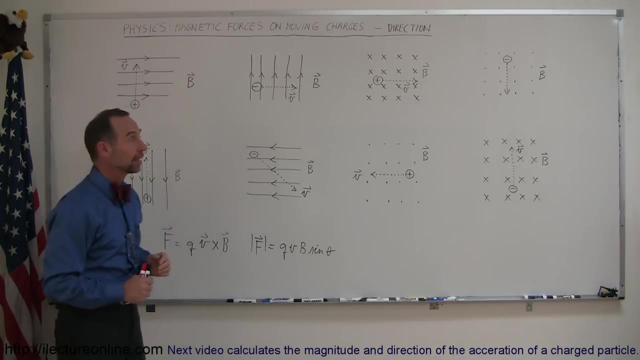 charges. you can see there's a charge here moving upward, charge here moving to the right, charge here moving to the right. also, notice that some charges are positive, some charges are negative and that does make a difference. now, the magnetic field is indicated by this b with an arrow on top. 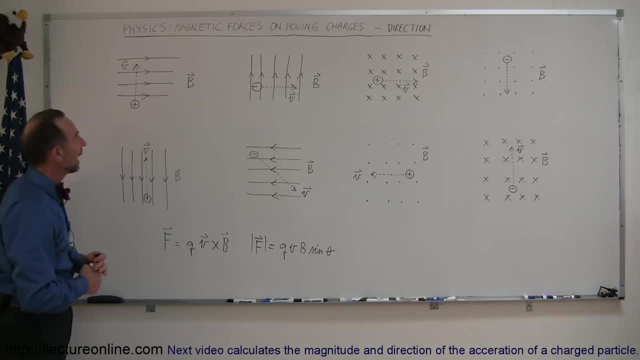 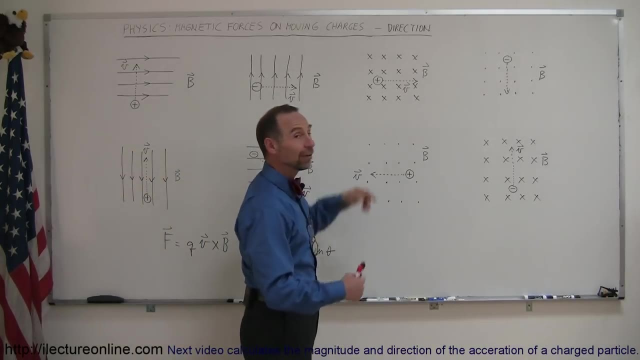 of it. so that's we sometimes call it the b, and the magnetic field is indicated by this b field or a magnetic field, and these arrows here are in the direction of the magnetic field. here the field is to the right. here it's up. this means that the field is into the board. it's like looking. 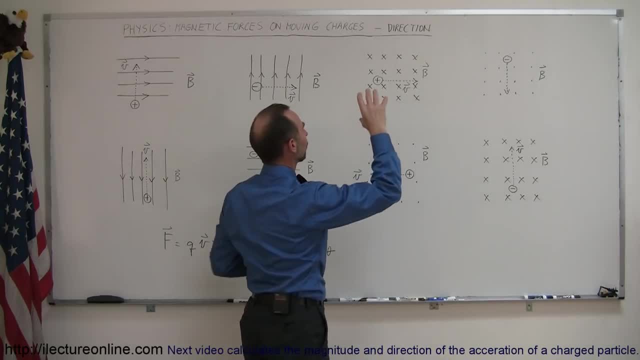 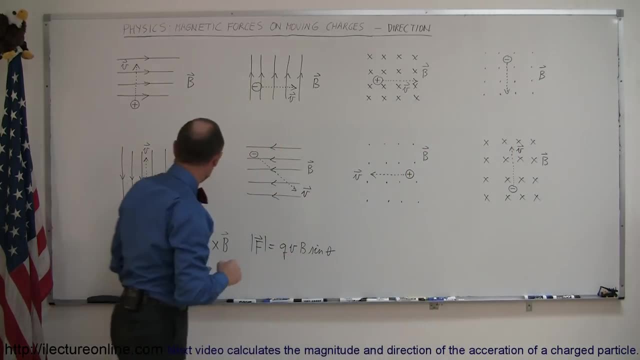 at the back of an arrow where you see the hairs in the back there. so the b field is into the board. here we're looking at the tip of the arrow, so the b field is out of the board, towards you. here again the field is downward, the field is to the left. here the field is out of the board. 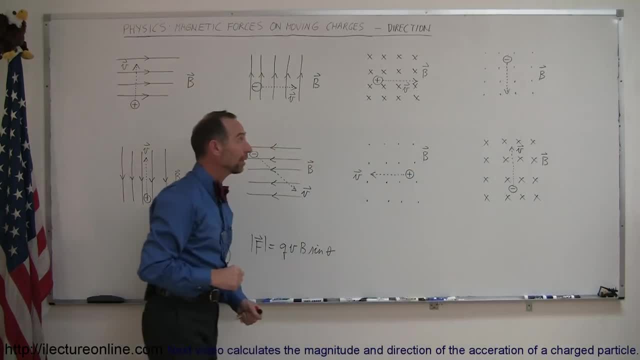 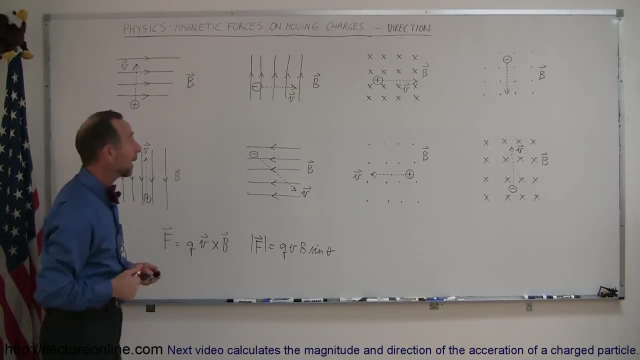 and there the b field is into the board. so, based upon that, what will be the direction of the forces of each of those eight charges in each of those eight different magnetic fields? and i'll use a red pen to try and indicate it the way that's. 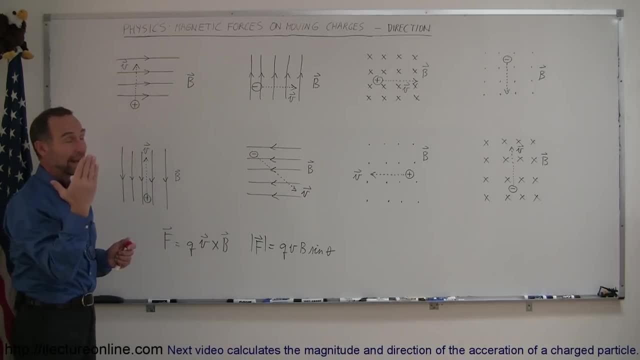 done is that if it's a positive charge, you use your right hand for the right hand rule. if it's a negative charge, you use your neck, your left hand for uh, for negative charges, to find the direction of the, of the force and uh. so how do you do that? well, you take 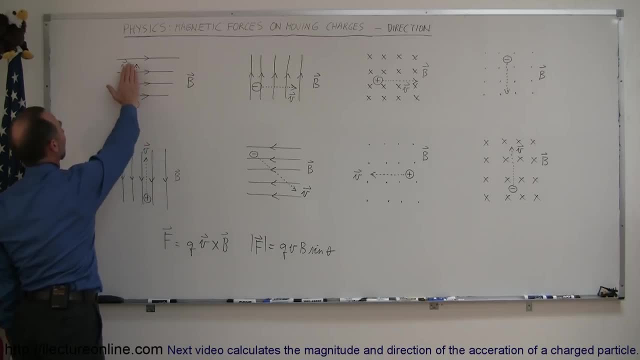 your hand and you point your fingers in the direction of the velocity of the charge, and since it's a positive charge, i'm using my right hand, like. so then you have to turn your hand whatever direction you need to, so you can curl your fingers in the direction of the b field. so i'm pointing upward and then i point this way to 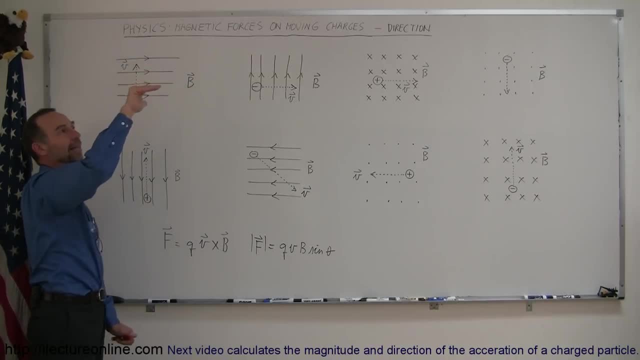 show the direction of the b field. so up for the velocity this way, the b field, and then my thumb points inward into the board so i can say: then the force- and i'll indicate that a little cross, the force then will be into the board. so velocity up b field this way, force into the board. looking at this example here, now of course i need 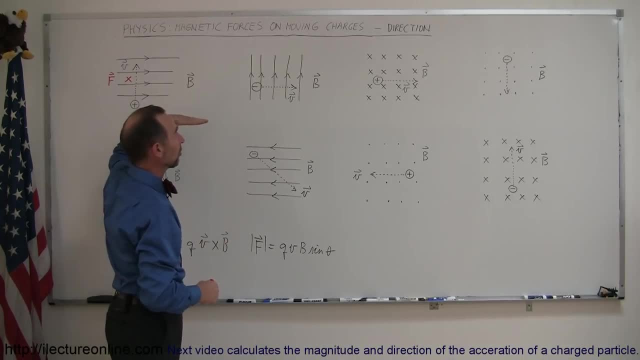 to use my left hand because it's a negative charge. i point my fingers in the direction of the velocity of the of the charge. then i have to curl my fingers in direction of the b field. of course i can't curl my fingers upwards. i have to turn my hand around. i cannot curl my fingers upward. 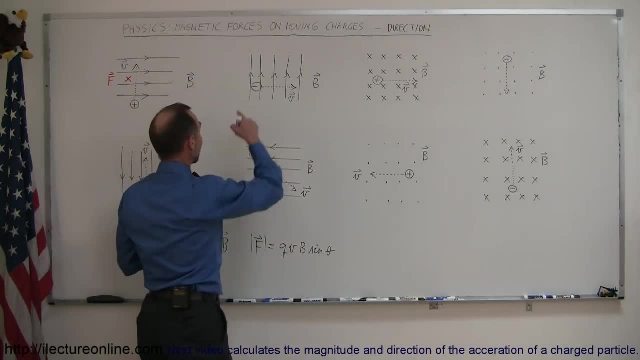 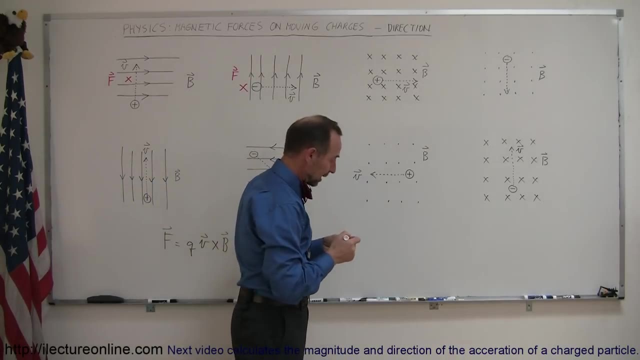 and my thumb points into the board. so here also, the force on this charge will be into the board. okay, going to our next example, here we have a b field that's into the board. but oh, i need to use my right hand because it's a positive charge. take my right hand, point my fingers. 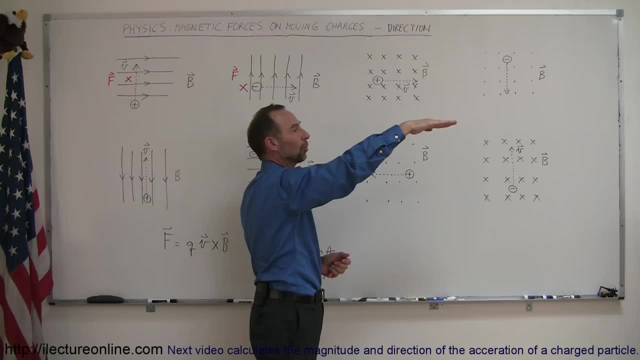 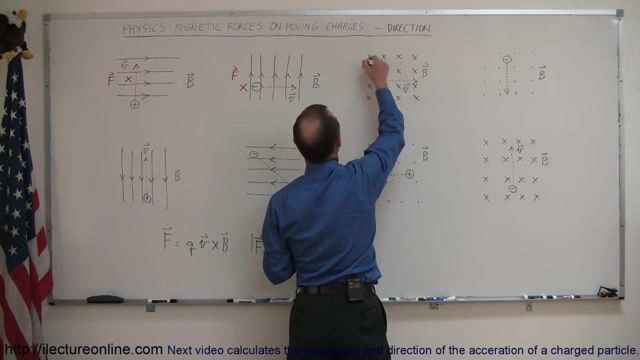 in the direction of the velocity of the charge. then i have to curl or turn my hand in such a way that i can curl my fingers towards the b field which is into the board, and now my thumb points upward. so i can see now that the force on this charge will be upward. so we can go like this force. 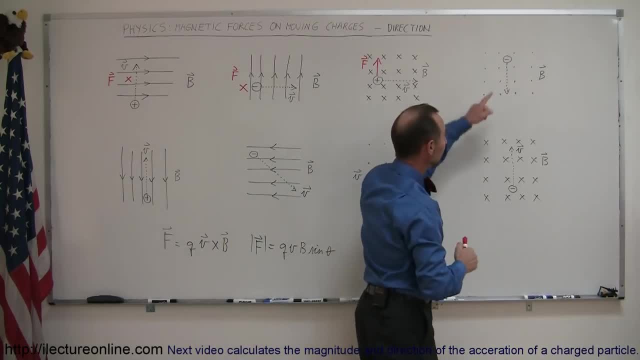 is upward, all right. next example: negative charge means i have to use my left hand. i point my hand in the direction of the velocity which is down. now i have to turn my hand in such a way that i can curl my fingers in direction of b field, which is out of the board. so i turn my hand around this way, point my fingers. 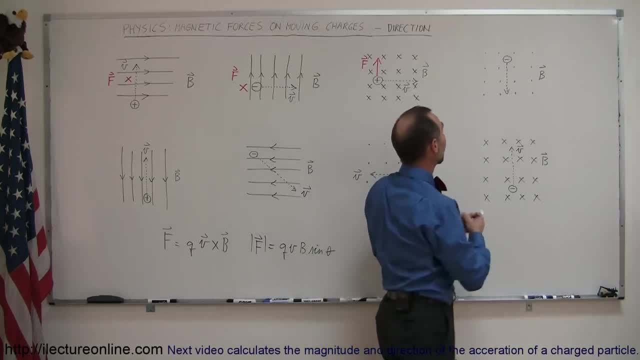 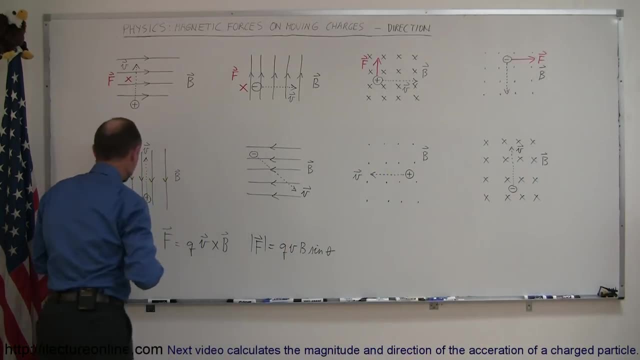 outward, and then my thumb points to the right, which means that the force on that charge will be to the right. all right. next example: here we have a positive charge, so i use my right hand, i point my fingers in direction of the velocity, which is upward. now i have to turn my fingers in the direction of b field, which is downward. ah, but. 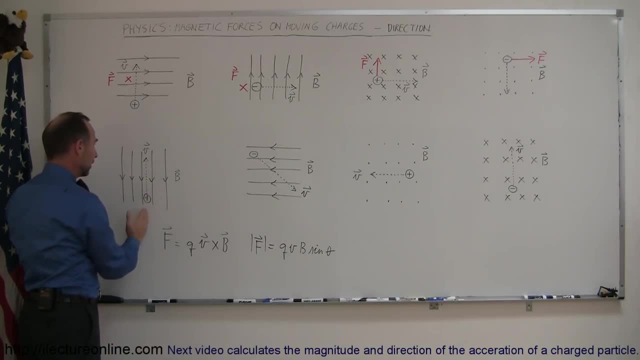 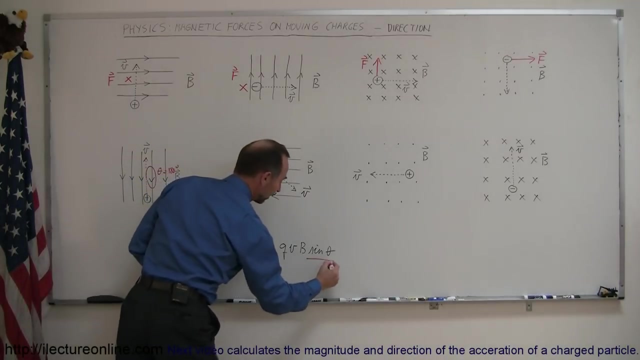 now we realize that the b field is down, the velocity is up. the angle between them is 180 degrees, so we have an angle here that goes from there all the way to here, which is theta equals 180 degrees, and of course the sine of 180 degrees is zero, and therefore 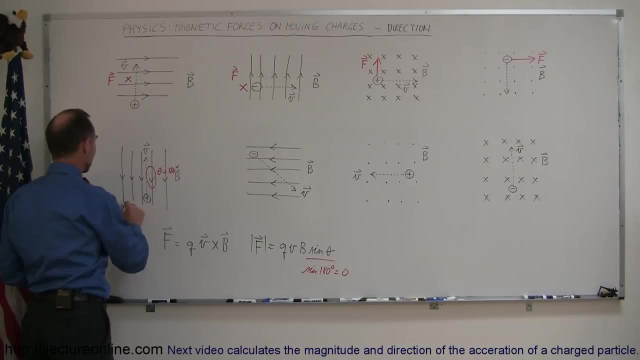 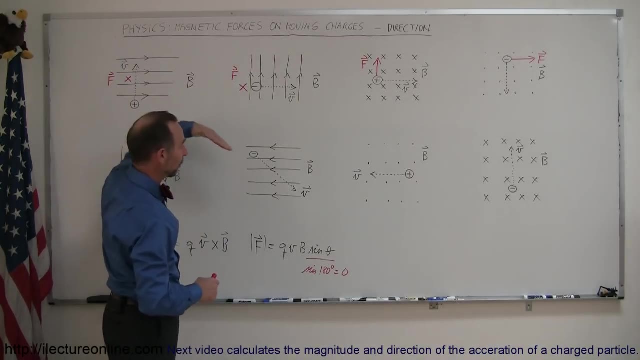 there's no force. so here we can say that force equals zero. no force on that one, all right. next errand: we have a negative charge. so i use my left hand, i point my fingers in the direction of the velocity which is down. now i curl my fingers in the direction of the b field, which 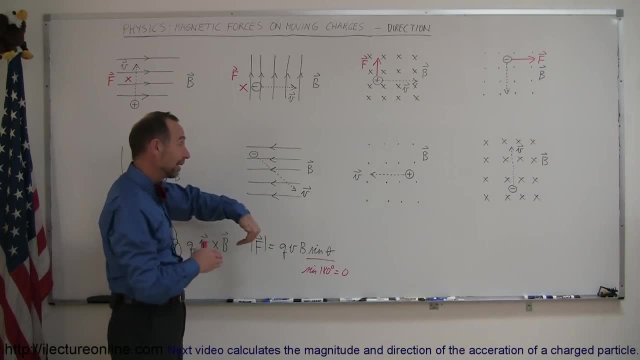 is this way. now, even though it's not a 90 degree angle, it's not a 180 degree angle, so the sine of something between 90 and 180 is still a valid number somewhere between zero and one. so i will have some sort of force. 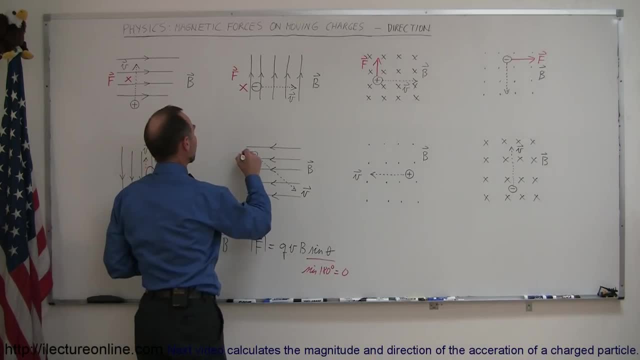 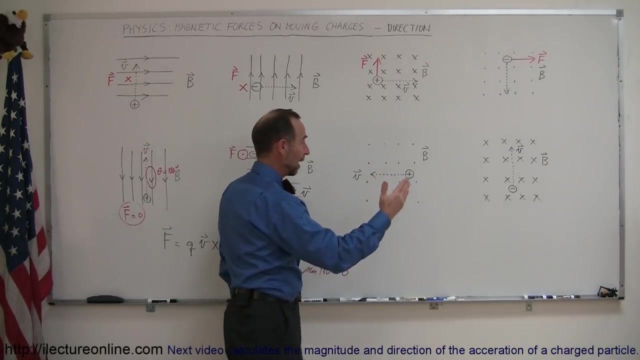 my thumb is pointing outward so I can say that the force on this charge will be outward. so force is out of the board. I indicate that with a dot. sometimes we indicated with that with a little circle around it like the tip of an arrow. all right now. next example: positive charge. I use my right hand, I point my fingers in. 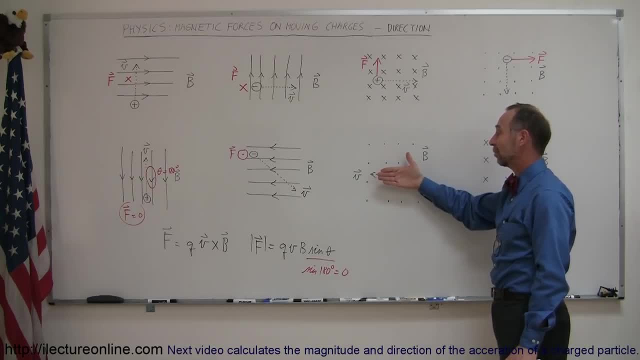 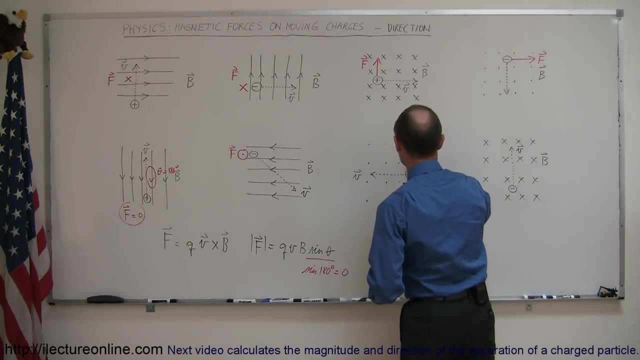 the direction of the velocity. and then I have to turn my hand this way so I can turn my fingers in the direction of the B field, which is out of the board, and the force in that case will be up. and finally, last example, here let me move. 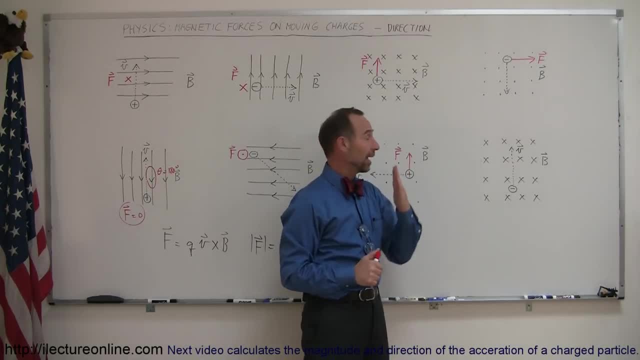 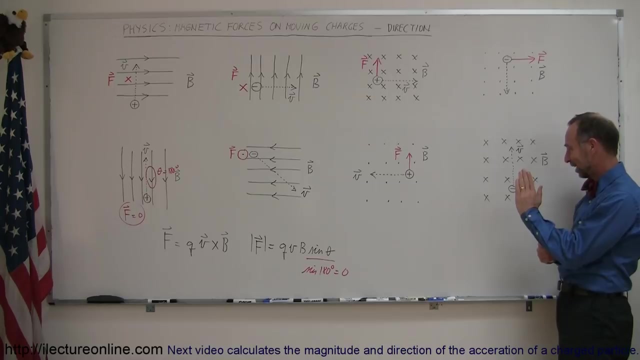 over. this way we have a negative charge. so we use left hand, we point our fingers in the direction of the negative, the velocity of negative charge. now I have to turn my hand in such a way. I guess I'll have to come this way sometimes. anatomically it's hard to do these things unless you stand correctly. so 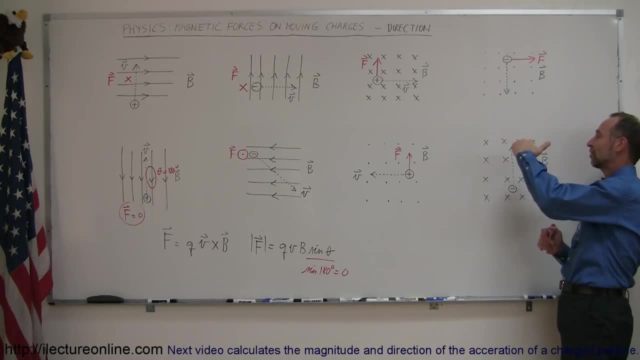 fingers in the direction of the velocity you then you point your fingers in the direction of B field, which is into the board and looks like my thumb is pointing this way. so this charge will feel a force in this direction there. so hopefully that clears it up for you. 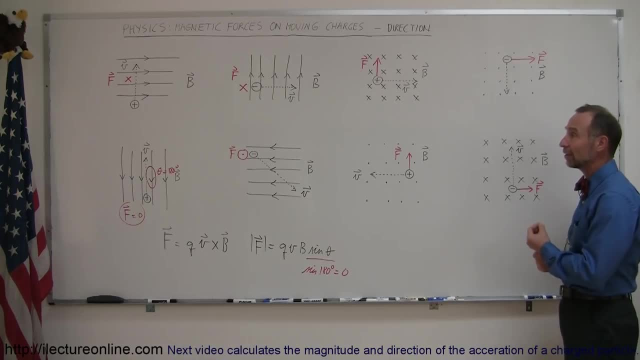 whenever you have a moving charge in a magnetic field, the charge will feel a force as long as the the direction of the velocity is not parallel with the direction of the magnetic field. and to find the direction of the charge, of the force on the charge, you use your right hand. 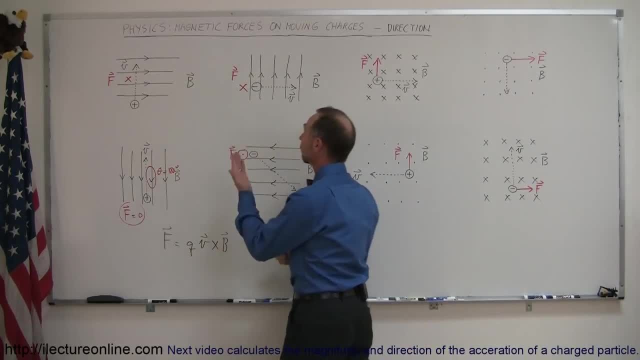 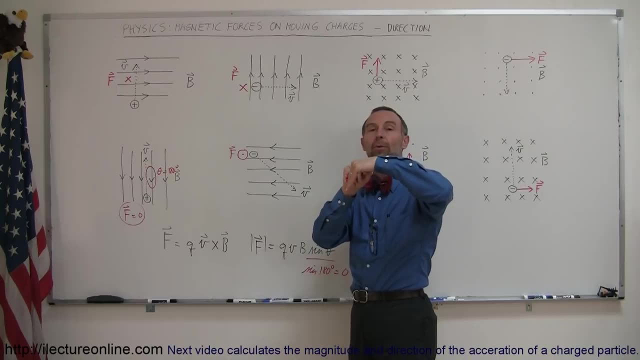 or use your left hand, right hand for positive charges, left hand for negative charges. point your fingers in the direction of the velocity, then curl your fingers in the direction of the B field. your thumb will point in the direction of the force. so that's called the left or right hand rule for finding the force. 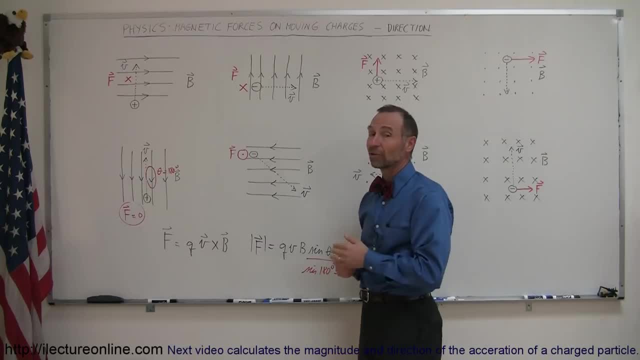 on the charge of the direction of the force on a moving charge in a magnetic field. all right, now we go on and actually start calculating some of the actual magnitude of these forces and direction of the forces in some examples coming up in the next video.